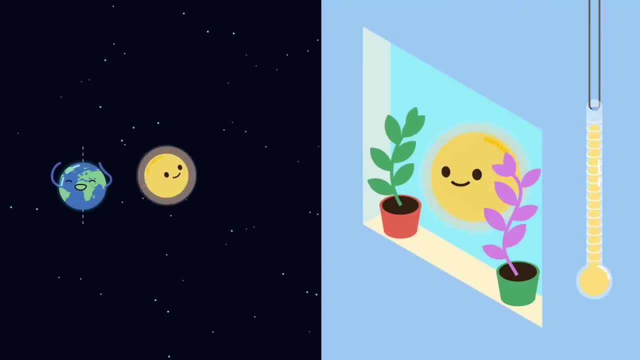 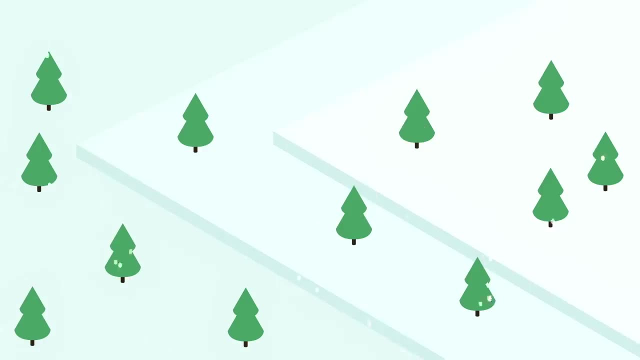 These wobbles, combined with the planet's elliptical orbit, cause summer temperatures to vary depending on whether the summer solstice happens when Earth is closer or farther from the Sun. Approximately every 100,000 years, these factors align to create dramatically colder conditions. 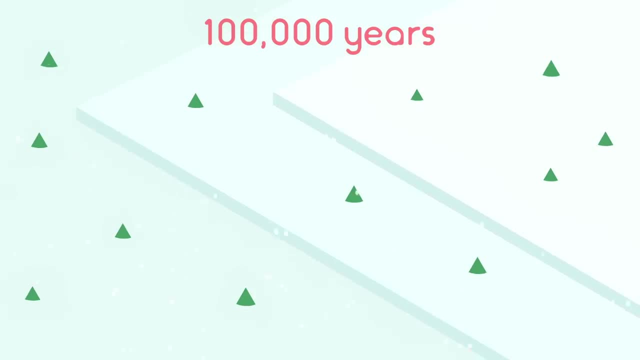 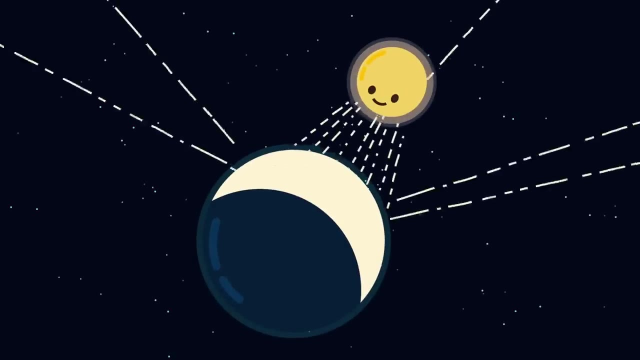 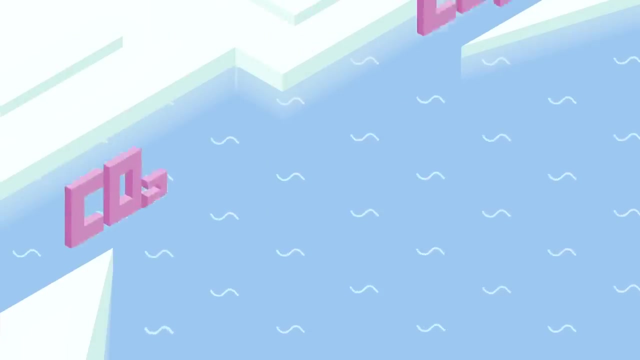 that last for millennia. Cool summers that aren't warm enough to melt the preceding winter's snow allow ice to accumulate year after year. These ice sheets produce additional cooling by reflecting more solar energy back into space. Simultaneously, cooler conditions transfer carbon dioxide from the atmosphere into the ocean. 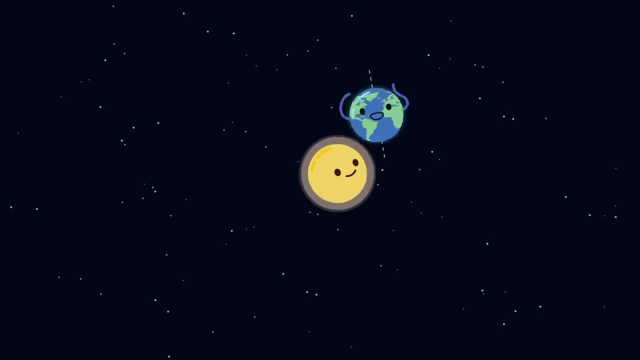 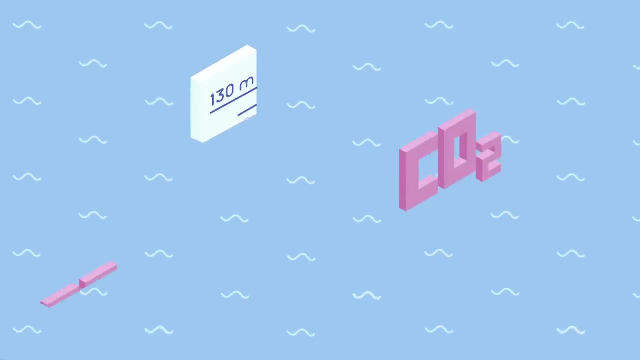 causing even more cooling and glacier expansion. About 20,000 years ago, these trends reversed when changes in Earth's orbit increased summer sunshine over the giant ice sheets and they began to melt. The sea level rose 130 meters and carbon dioxide was released from the ocean back into the atmosphere. 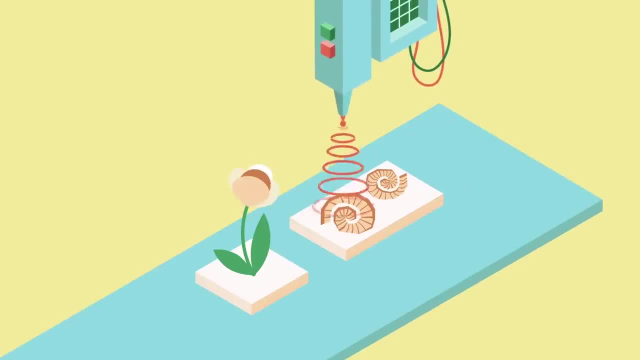 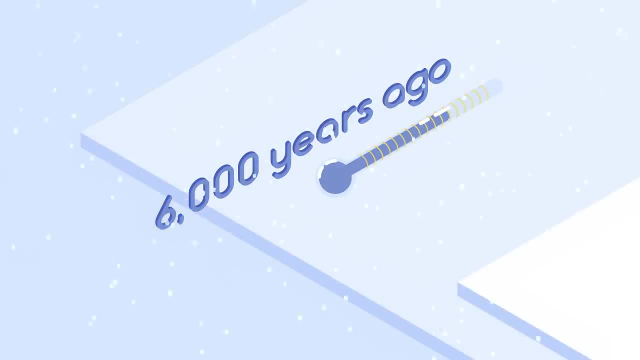 By analyzing pollen and marine fossils, geologists can tell that temperatures peaked about 6,000 years ago, before another shift in Earth's orbit caused renewed cooling. So what's coming next? Based on the repeated natural cycles seen in the climate record, 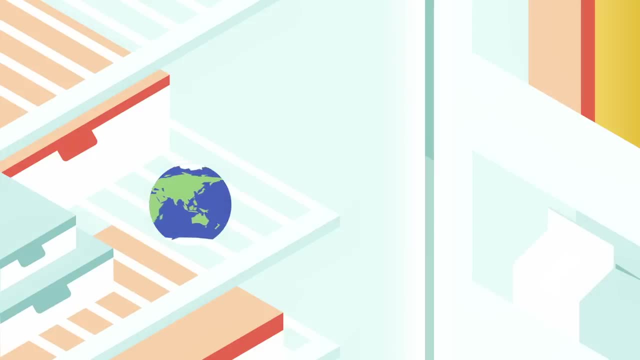 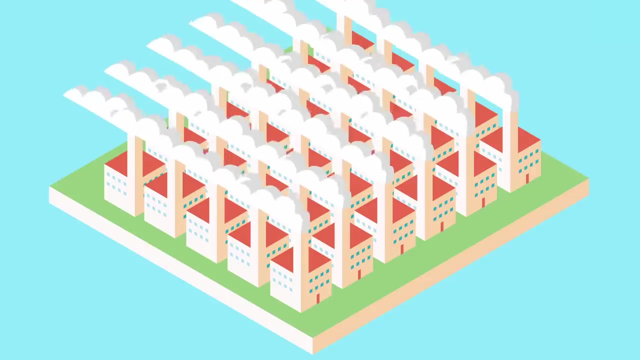 we'd normally expect the Earth to continue a trend of gradual cooling for the next few thousand years. However, this cooling abruptly reversed about 150 years ago. Why Carbon dioxide levels in the atmosphere have been rising since the 19th century, when fossil fuel use increased. 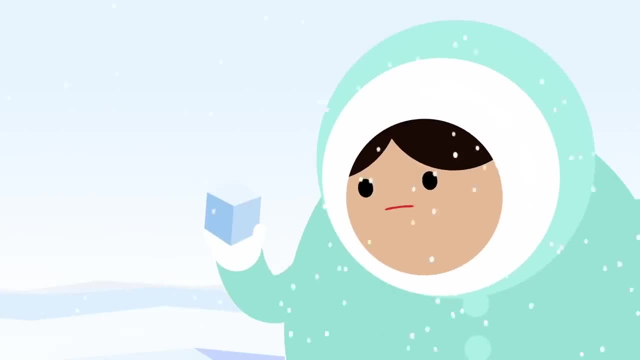 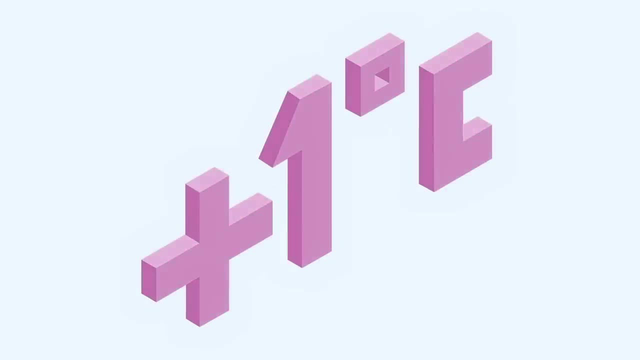 We know that from studying air bubbles trapped in Antarctic ice. This surge in carbon dioxide also coincides with a global temperature increase of nearly one degree Celsius. Ice cores in atmospheric monitoring stations show us that carbon dioxide levels are rising faster and to higher levels. 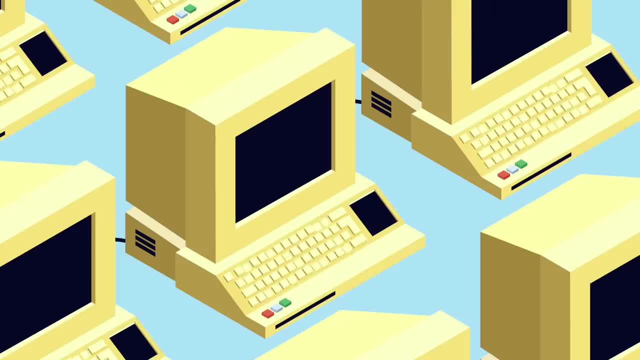 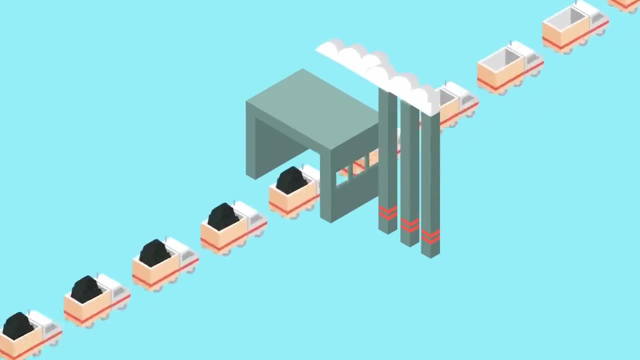 than at any point in the last 800,000 years. Computer models forecast another 1 to 4 degrees Celsius of warming by 2100, depending on how much additional fossil fuel we burn. What does that mean for the ice currently on Greenland and Antarctica? 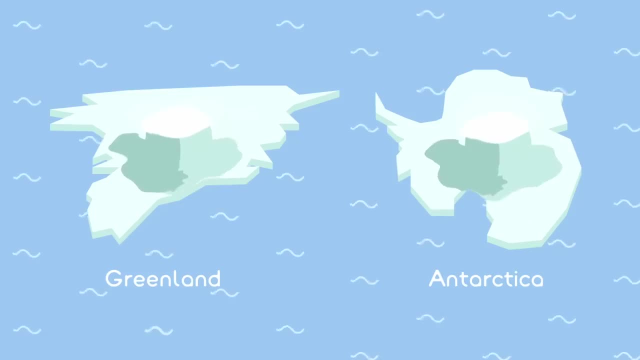 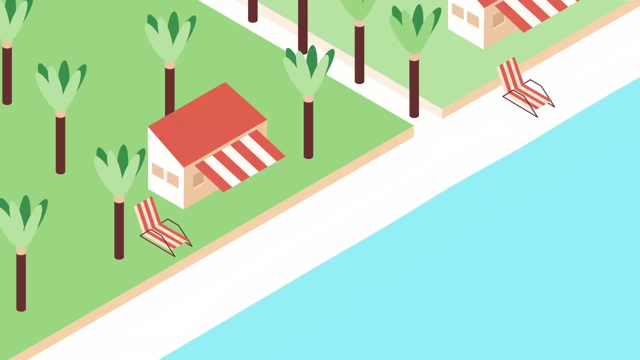 Past climate changes suggest that even a small warming shift can begin a process of ice melt that continues for thousands of years. By the end of this century, ice melt is expected to raise the sea level by 30 to 100 centimeters, enough to impact many coastal cities and island nations.